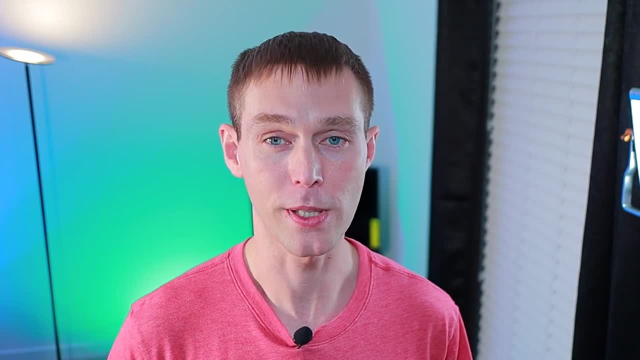 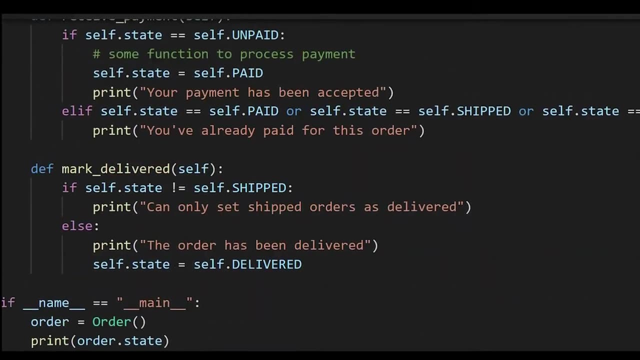 Let's look at the code that has a potential to be converted, to use the state pattern. Here we have an order class that has a few methods, and in each method we print something different depending on the current state of the order. As you can see, there is a lot of if and elif. 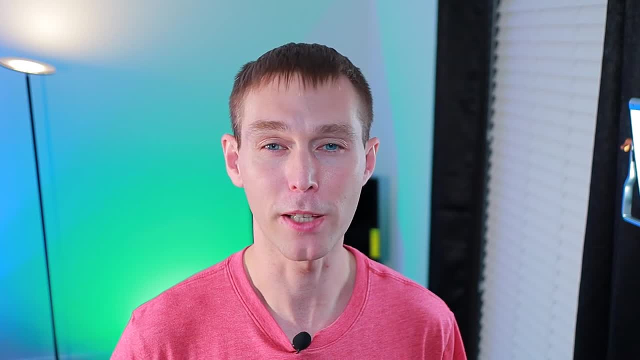 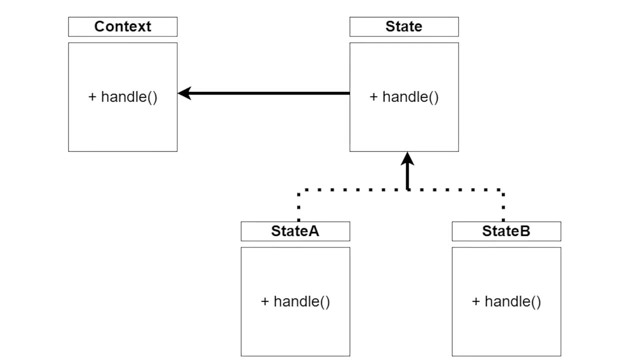 statements. This makes our class very hard to modify and very prone to errors, especially if you don't have an existing unit test coverage. Here is the diagram of the state pattern. It's actually a little bit more complicated than the previous one, but it's a little bit more. 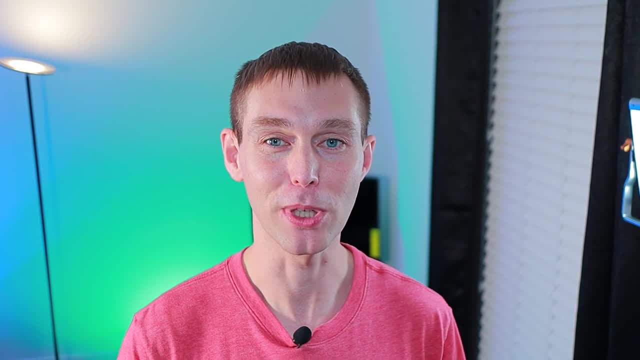 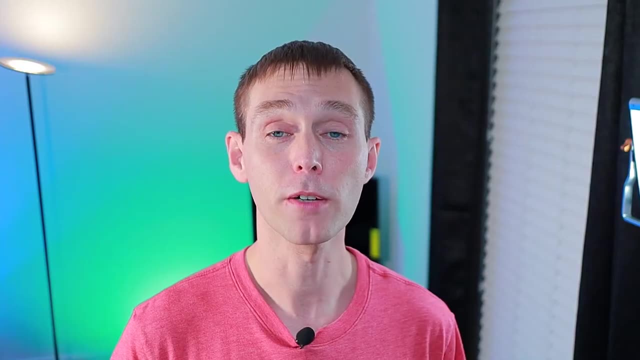 really simple. A state is just that. A state, an object, can be in More states. an object can be in more implementations of the state interface. we will have to write: What about the context? Think of a context as a state of states. It represents our 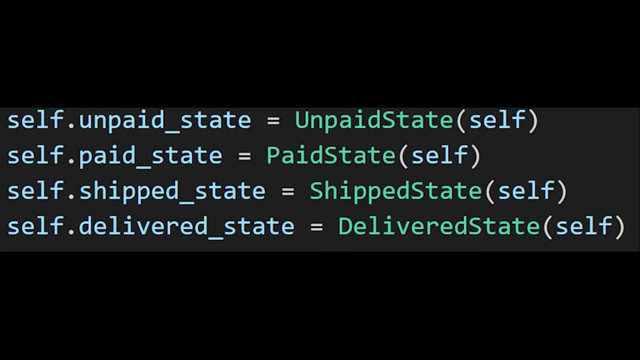 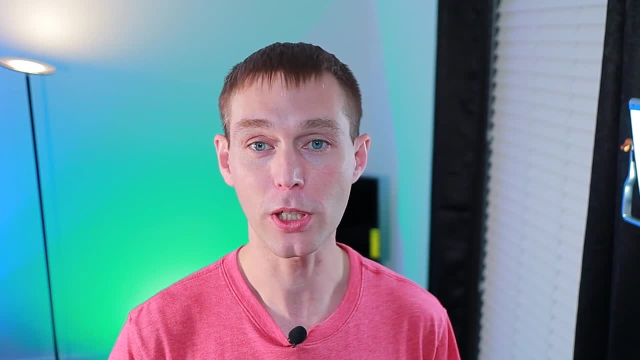 object's current state, as well as stores other states an object can be in. So in our case, order class would be the context. Now let's see how we can convert the existing order class to use the state pattern. First let's define which methods should be on our interface. 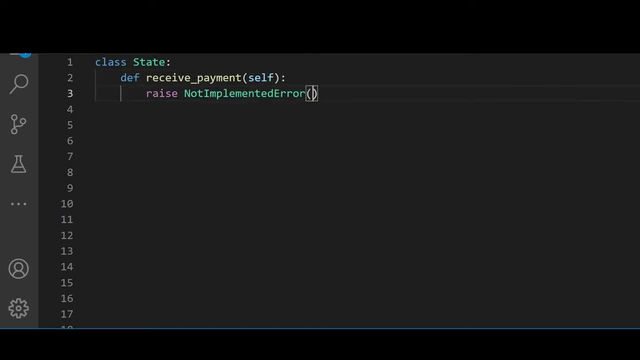 In our case, it's going to be the same methods we have on the order: class: Receive, payment, ship and mark deliver. Now we need to define which states we will implement in their own classes. That's pretty easy as well. It's all the states the order was already keeping track of. So 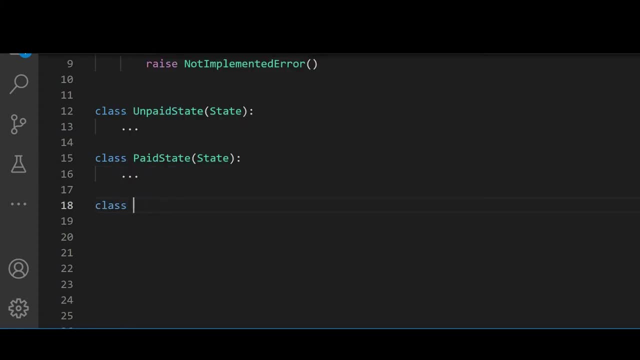 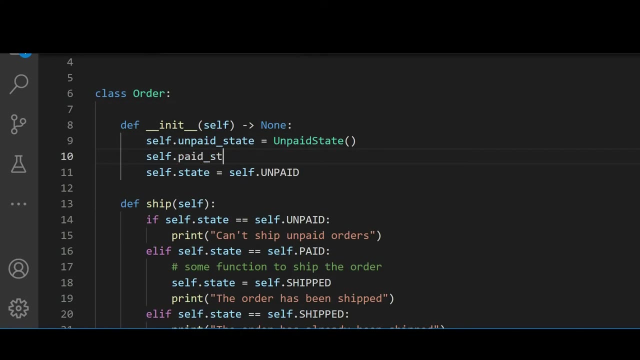 we will have unpaid state, paid state, shipped state and delivered state. Before we put any logic in them, we need to make a few changes to the order class. Let's replace our state variables from using integers as state to using the newly created state classes. Also, let's add a new state. 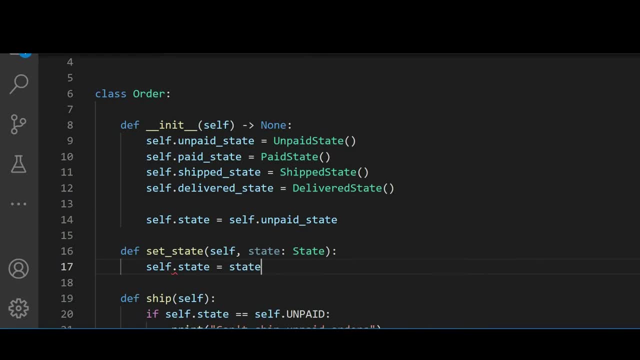 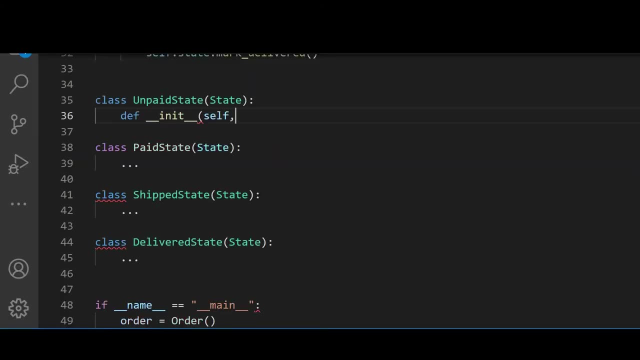 method so we could handle the state changes. Now let's implement our state classes based on the logic in the order class. Let's start with the unpaid state. First we'll need a reference to the context of the order object so we could change the state if needed In the receive payment. 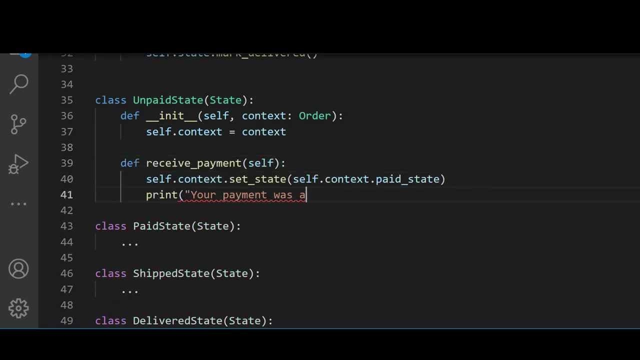 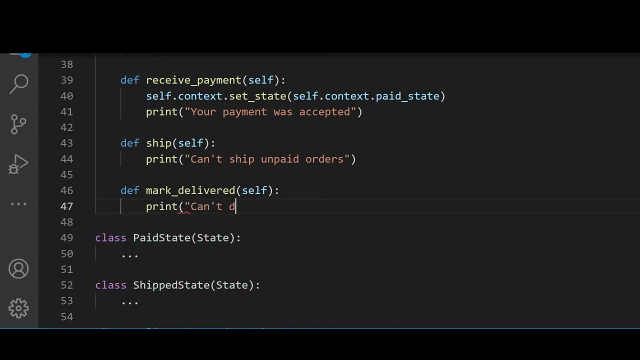 we can change the state to paid and print the message that the payment was accepted. Now in the ship function we just print that we can't ship unpaid orders And in the mark delivered function we say that we can't deliver orders that aren't shipped, And we repeat the same process for the